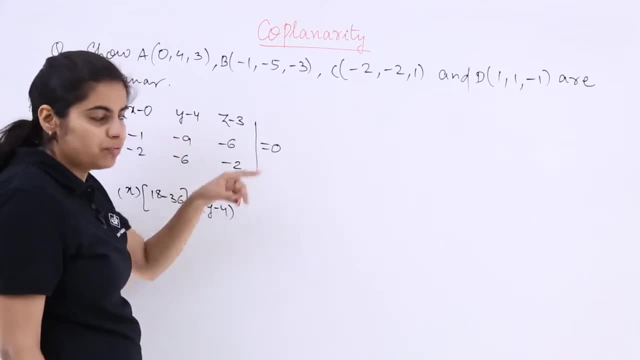 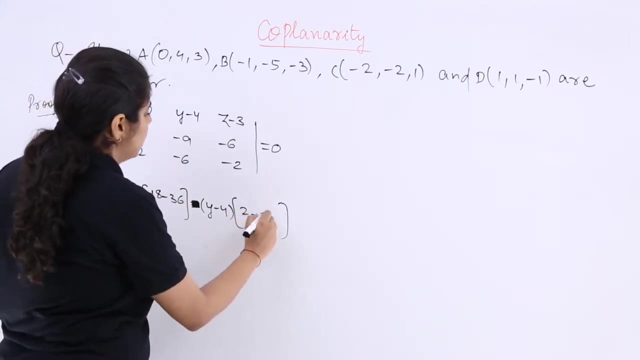 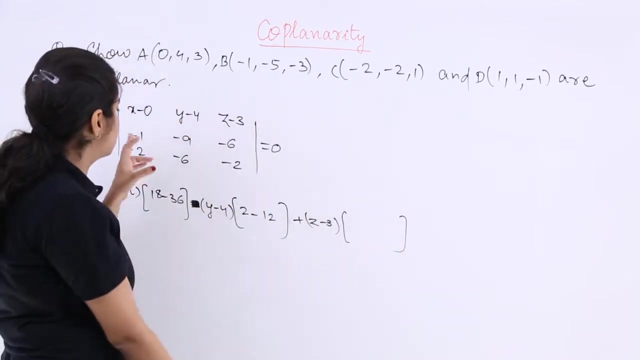 this should not be plus. This should rather be minus, because this is according to the cofactor convention. Remove the second column and the first row. It becomes 2 minus 12 plus z minus 3.. Remove the third column and the first row. It is 6 minus 18 is equal to 0.. 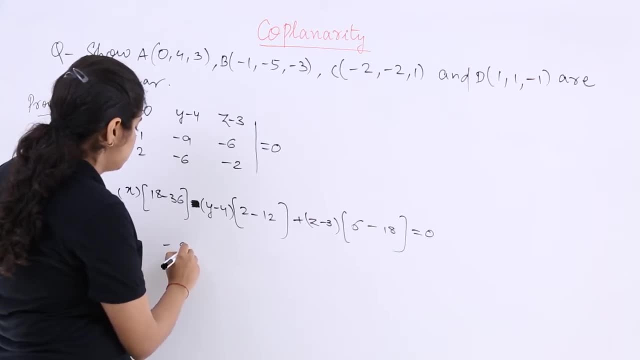 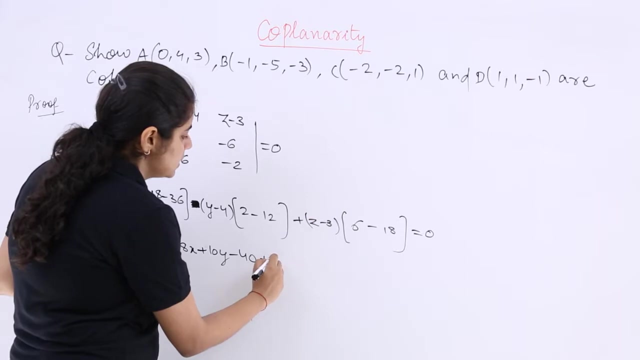 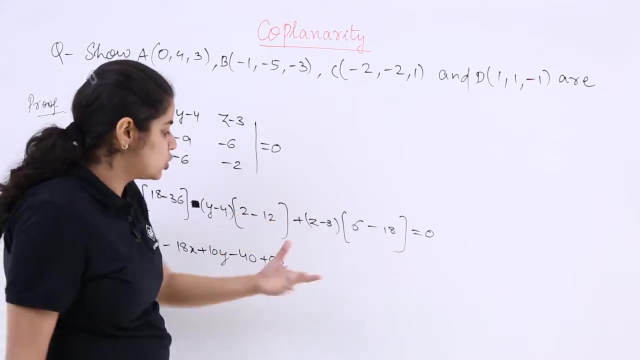 Right, So this is minus 18. multiply by x. Did I get it correctly, right? Wow, Yes, Then this is minus 10 into minus y, which is plus 10y. minus 10 into plus 4 is minus 40 plus 6z, right, minus 18z. so 6 minus 18 is minus 12. directly you can do minus 18z, which is 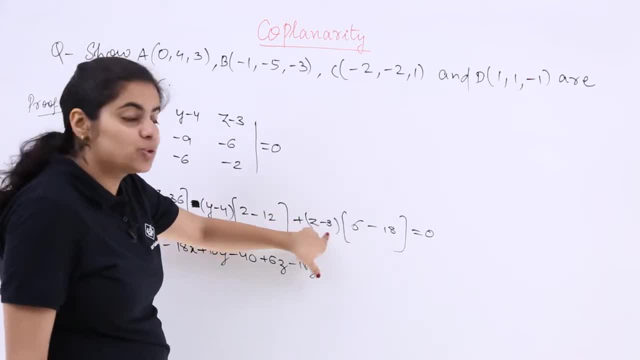 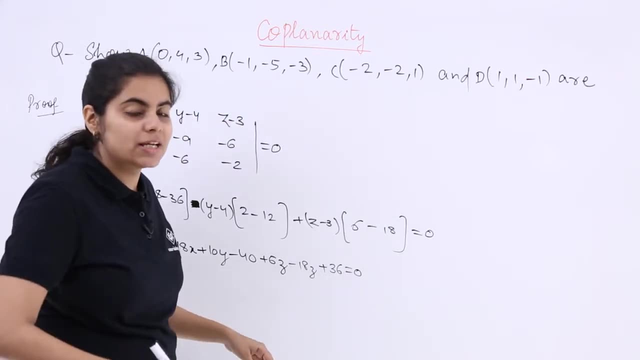 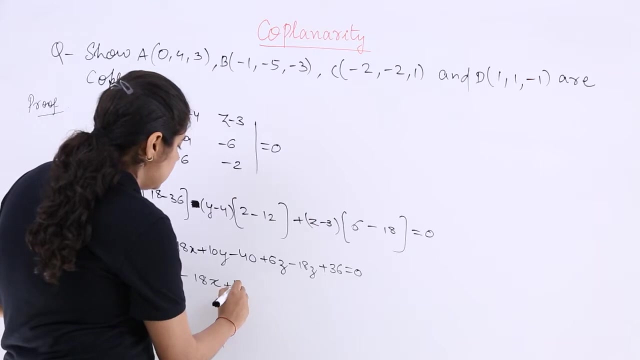 minus 12z, then this is minus 12 into minus 3, is plus 36, is equal to 0.. Now, wherever you have the constants, just make them one side and the other things to the other side. So it is minus 18x plus 10y, minus 12z, minus 4 is equal to 0. this is the obtained equation. 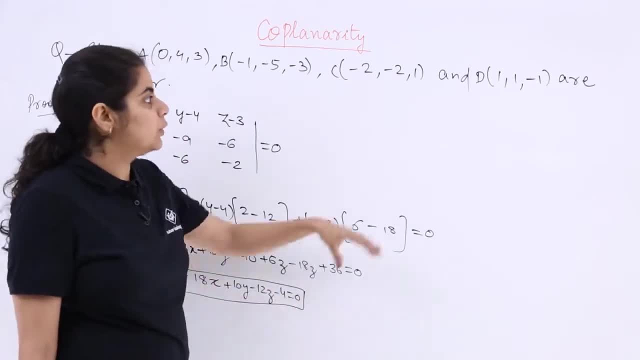 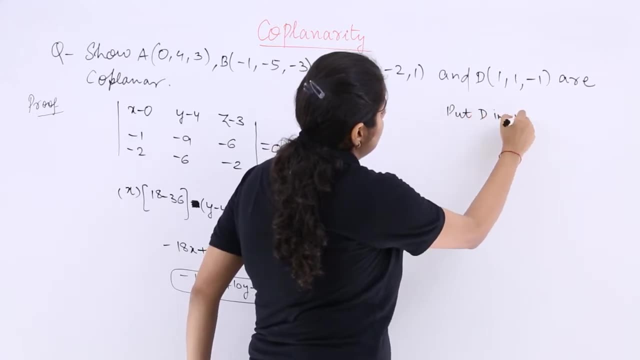 of a plane. Now, in order to check for coplanarity, just try putting the fourth point in this equation of a plane. So I write this as equation number 1. so you write: put d in equation number 1, so 1, 1 minus. 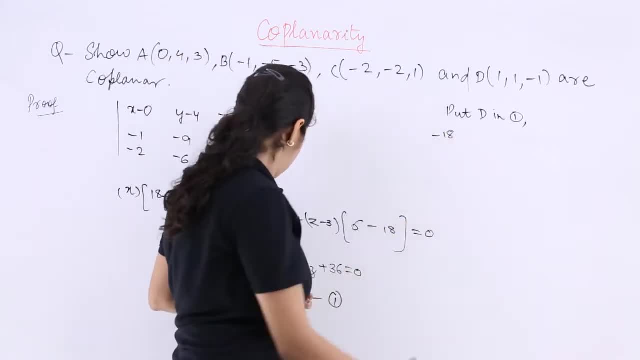 1. Putting 1, it is minus 18. putting 1, it is plus 10. putting minus 1, it is plus 12. having minus 4, it is minus 4. this is the LHS of the equation number 1. let's see whether it is. 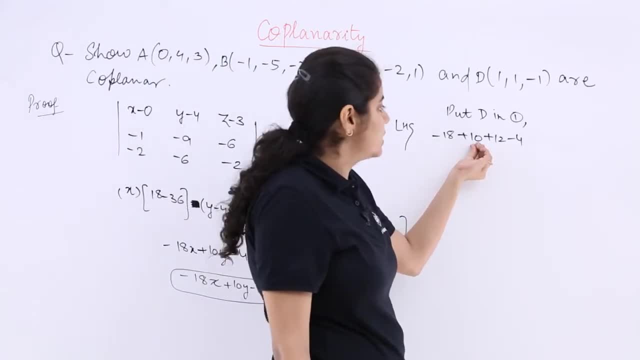 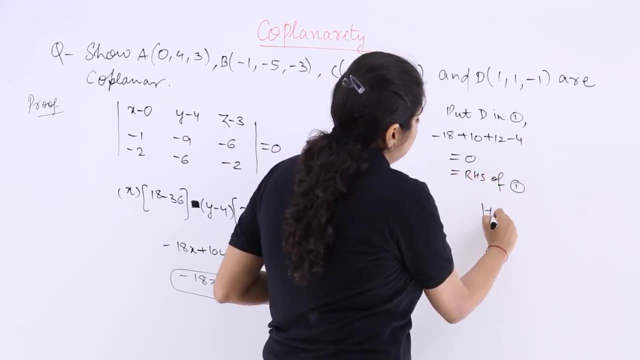 equal to the RHS, which is 0 minus 18 plus 10 is minus 8. minus 8 minus 4 is minus 12. minus 12 plus 12 is 0, which is equal to RHS of equation number 1. so that means the points. 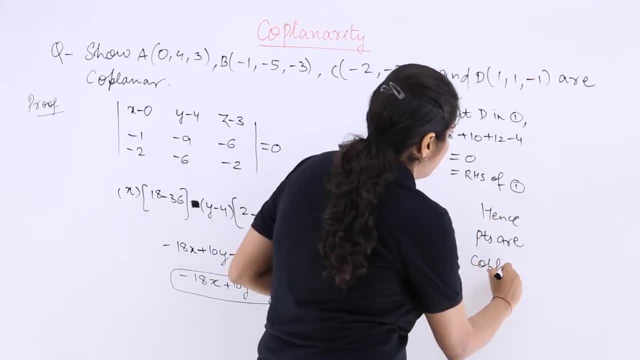 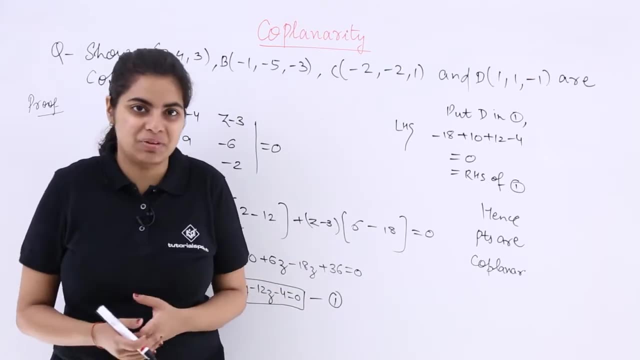 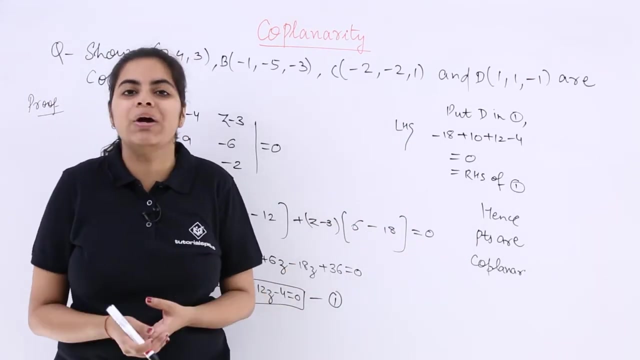 are Coplanar because for coplanarity only, we are going to see that three points have to be giving me an equation, and then the fourth has to be satisfied. so this is how we have to do it. so first we are going to solve this, find an equation, and then put the last remaining. 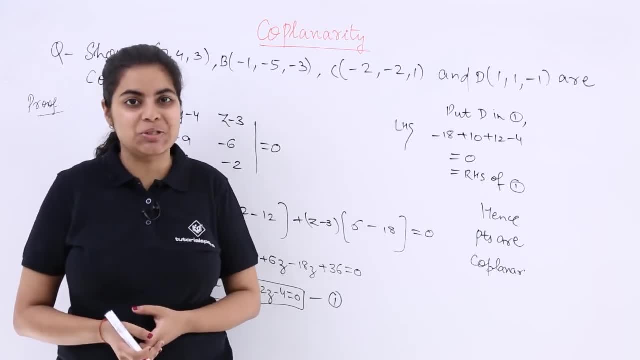 point in that equation: if it satisfies, it is coplanar, else it is not.